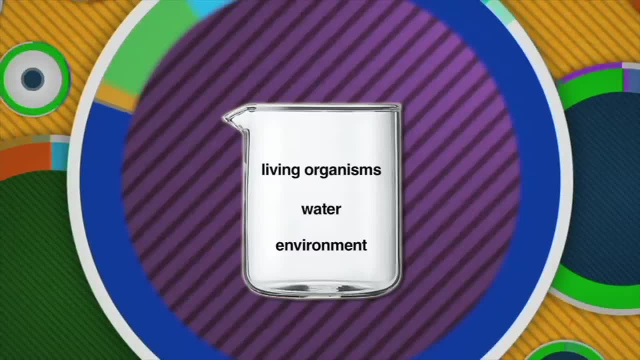 together to help maintain the other. There's another ecosystem: the living things that can act as��ies for each other and touching the level of their phones. Well, in fact, I don't need numbers to make this work, so take a really good look and 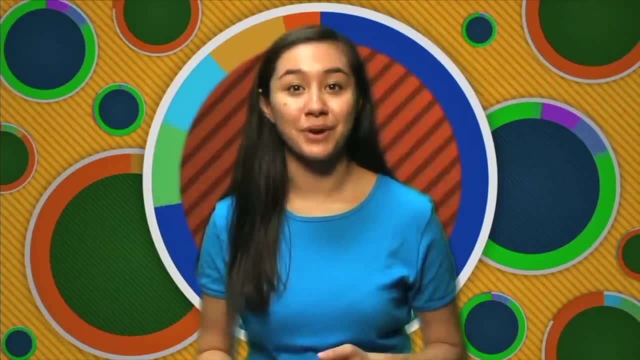 do your homework. The otter is an ecosystem just like you around Ecosystems that move about. when oneelles move the other and living things move around. when the other travels problems, they encounter times and forms similar to oneing things. 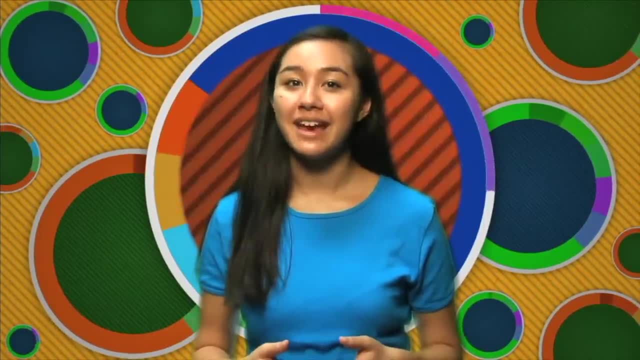 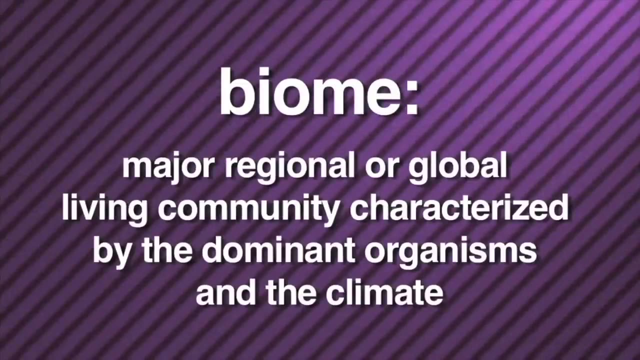 Here's a big picture of ecosystem. To understand what ecosystems this is, let's start with an ecosystem: organisms. These areas are called biomes. By definition, a biome is a major regional or global living community characterized by the dominant organisms and the climate. 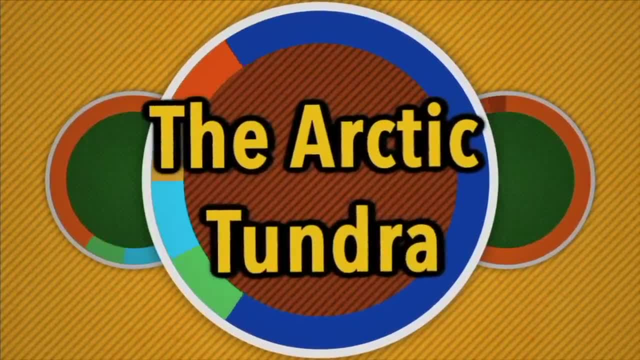 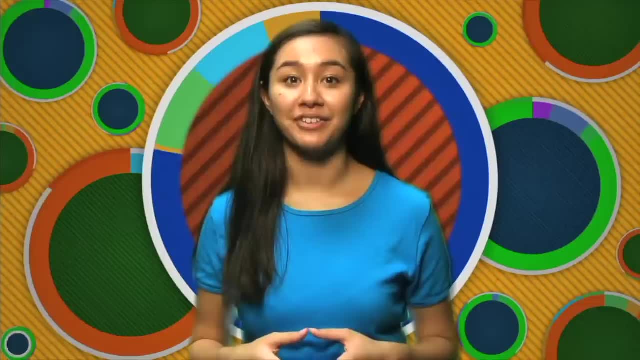 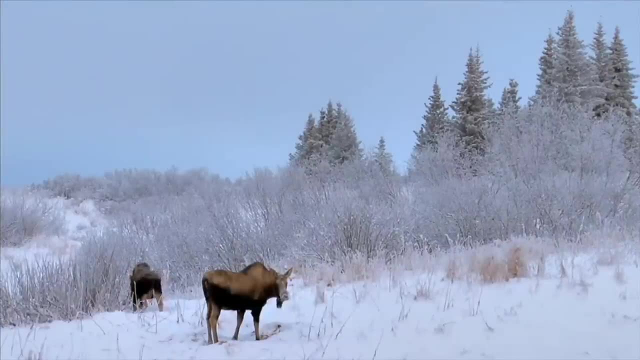 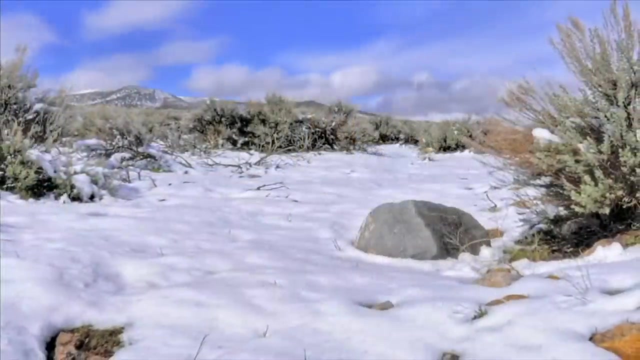 The Arctic tundra. In this program we are going to cover seven major biomes found on Earth. Let's begin with a biome we call the Arctic tundra. When you hear the word Arctic, you probably think of something cold. Well, you're right on track. The Arctic tundra is definitely cold, with temperatures. 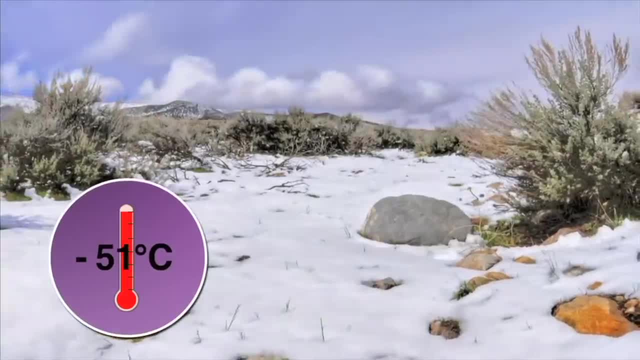 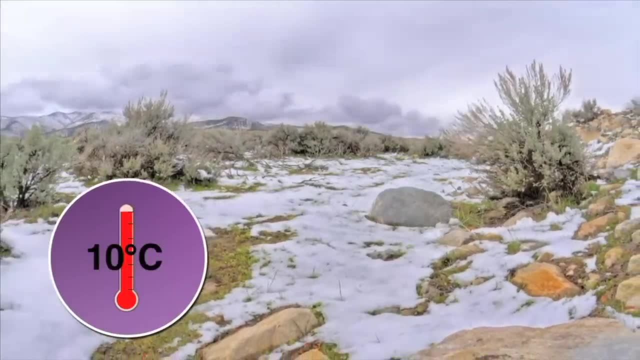 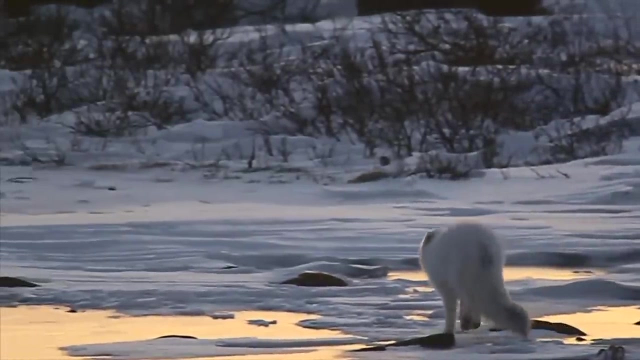 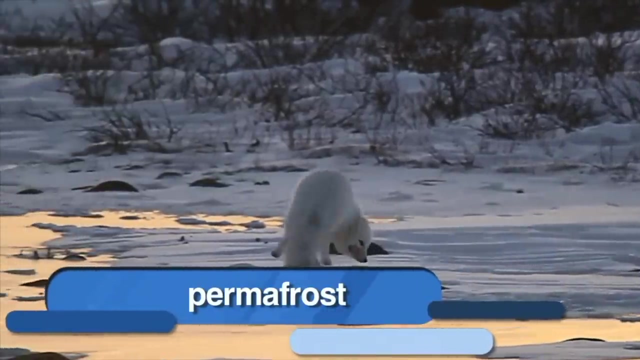 reaching almost negative 51 degrees Celsius during the winter. Even in the warmest months, the temperature rarely goes above 10 degrees Celsius Because the temperatures are so cold. the subsoil of the Arctic tundra remains frozen all the time. This permanently frozen ground is called permafrost, The 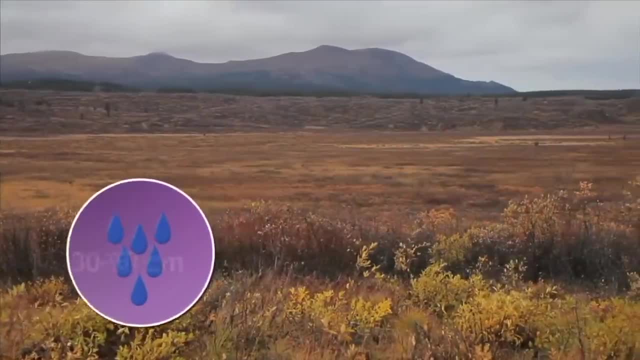 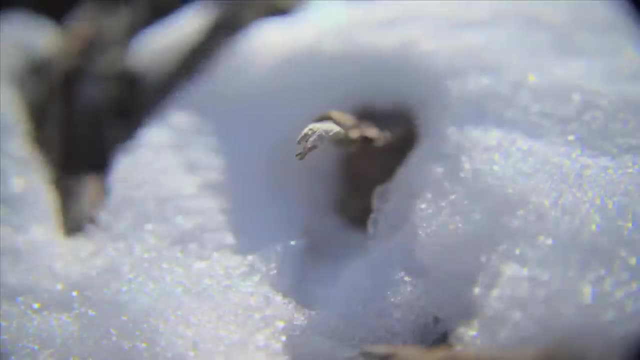 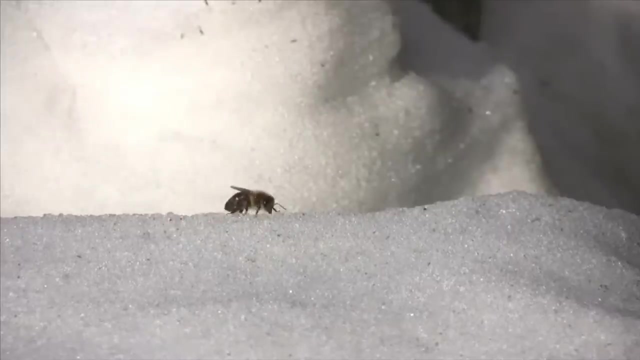 Arctic tundra has a mostly dry climate and sees between 30 to 50 centimeters of rainfall annually. During summer, it gets just warm enough for a thin layer of top soil to thaw and pools of water to form attracting insects, And some of those insects become 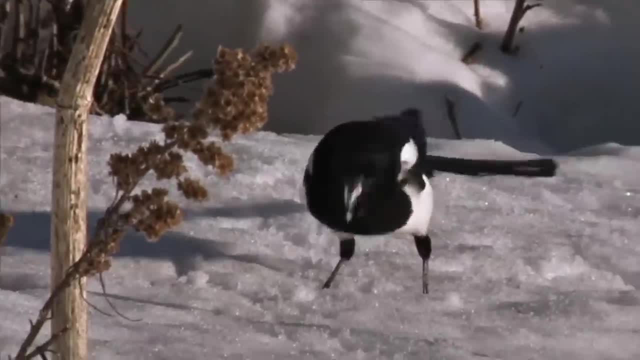 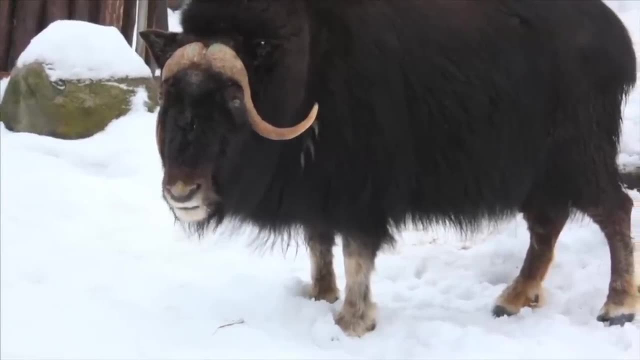 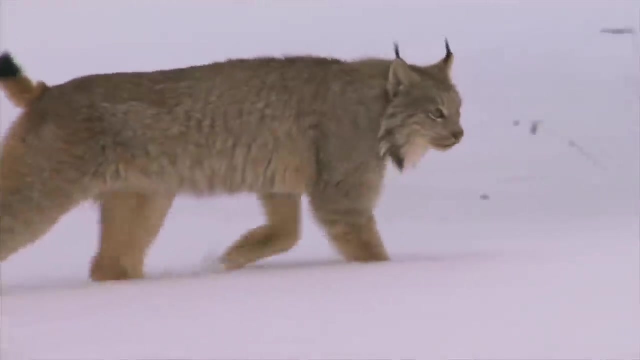 a feast for hungry migrant birds that venture into the area during that time of year. Throughout the rest of the year, however, the climate is extremely dry and cold, So the plants and animals that live there have special characteristics that help them survive in the environment. For instance, many of the animals that live 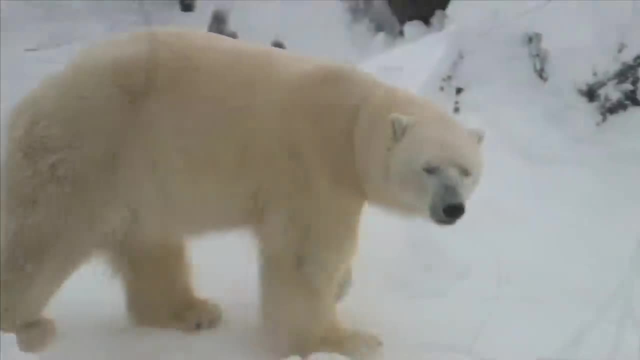 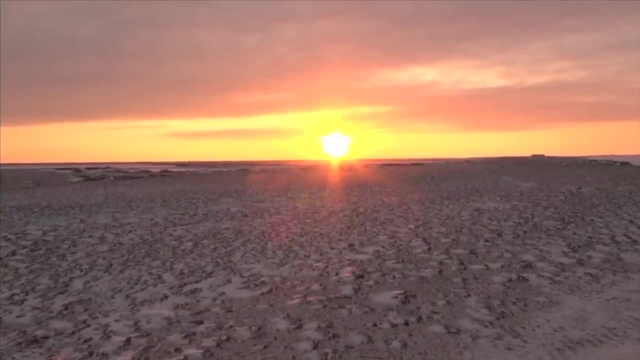 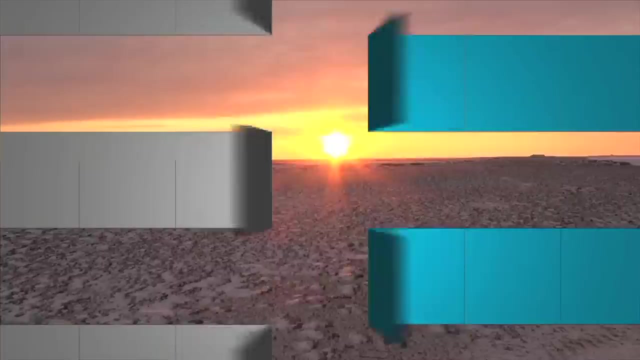 in the tundra have very thick fur Like polar bears, And you won't see trees in this area. They just can't adapt to the harsh conditions, So small shrubs and lichens are the dominant plants here. The Arctic tundra is the Earth's coldest biome and can be found mostly in the 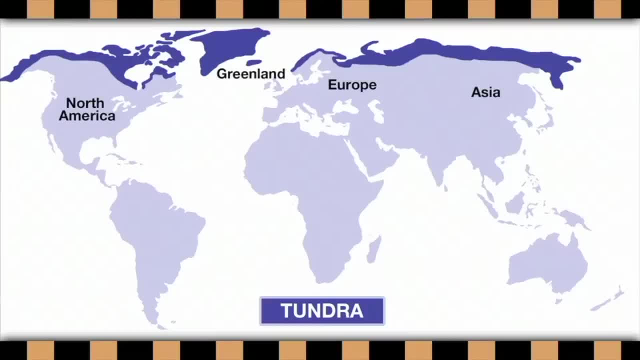 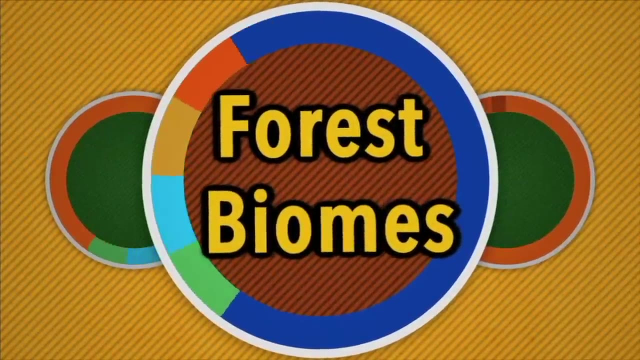 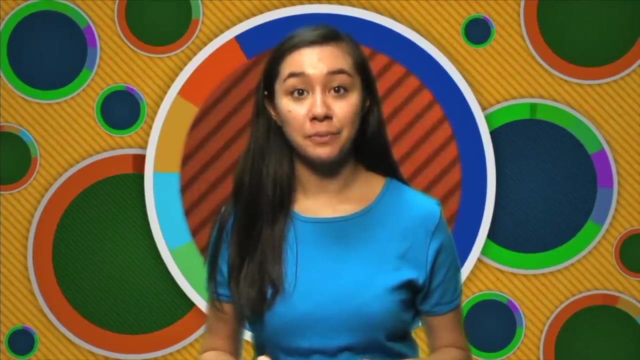 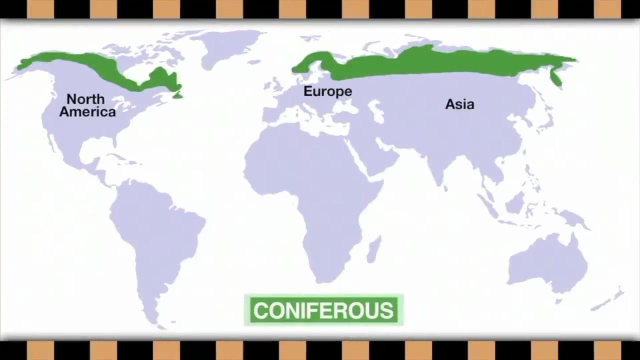 northern parts of the world near the Arctic Ocean and include lands in Europe, Asia and North America Forest Biomes. Just south of the Arctic tundra you can find a very different biome called the coniferous forest. The coniferous forest biome stretches across Alaska, the top of 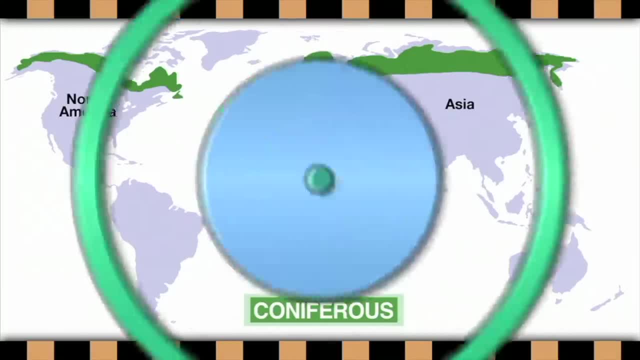 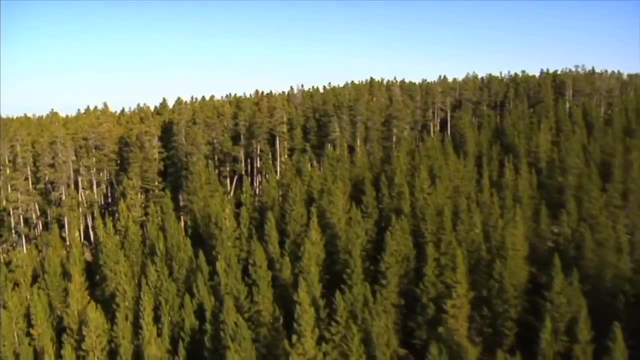 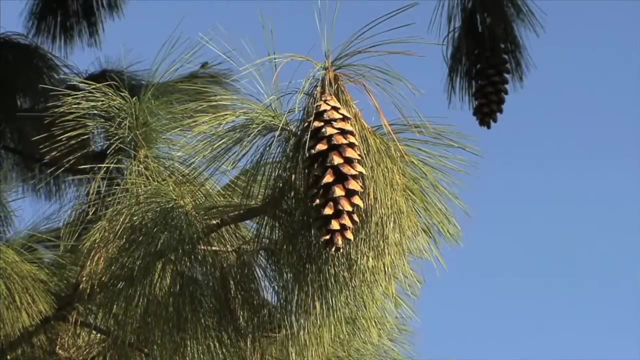 North America and Eurasia. What characteristics comprise the forest biome? Well, for one thing, you'll find plenty of trees here. The coniferous forest consists of cone-bearing trees with needles like spruce, henlock and firs. These trees don't have 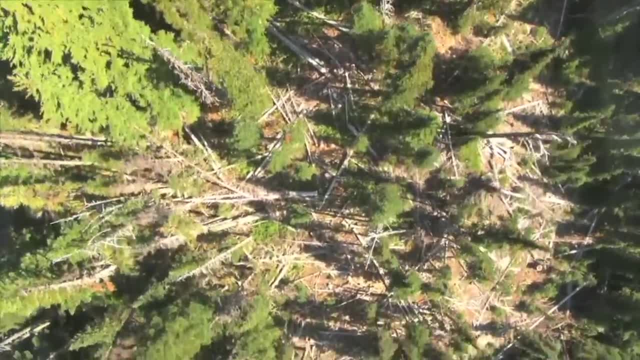 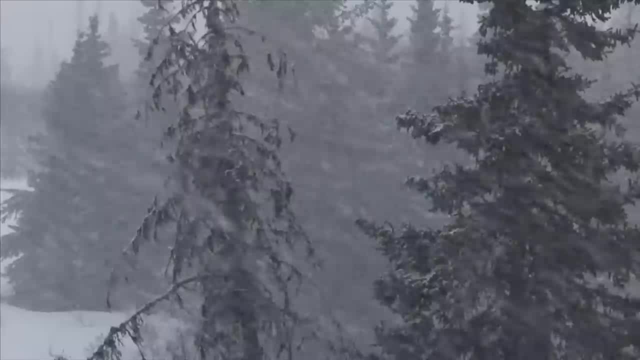 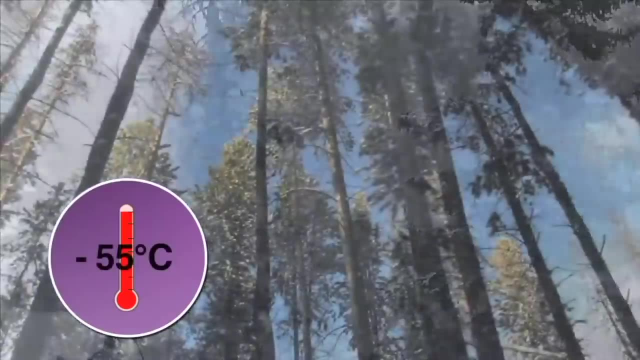 leaves that fall off and decay, so the soil in the coniferous forest is not very fertile. But the coniferous trees grow well here and are suited to the cold climate of this area, which has temperatures ranging from negative 55 degrees Celsius in the winter and up to 20 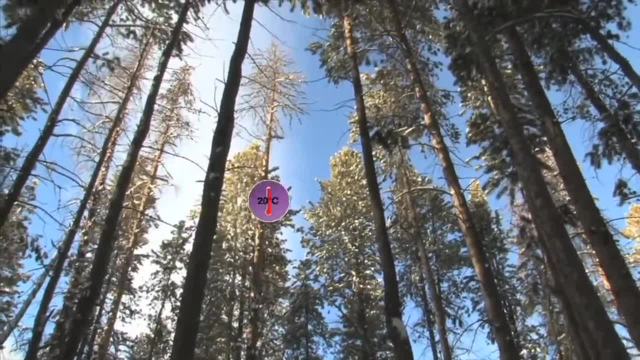 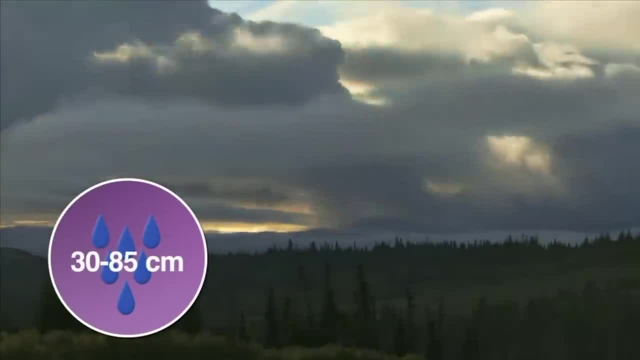 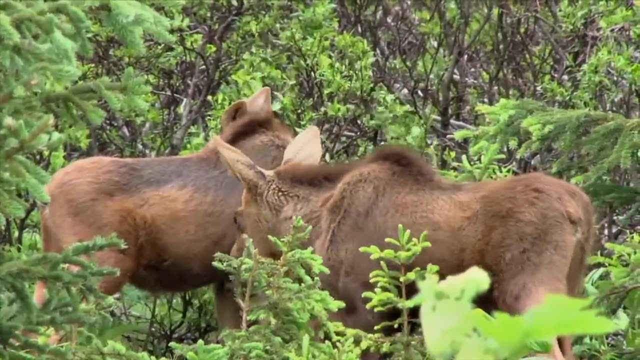 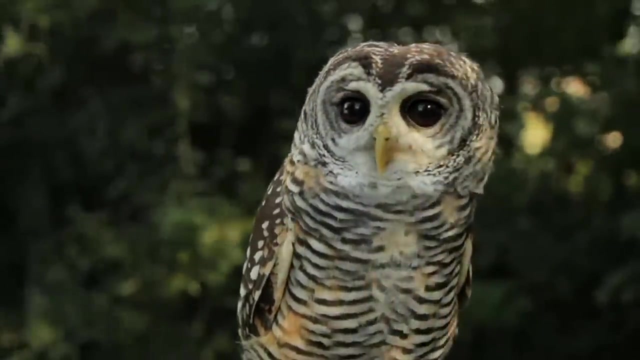 degrees Celsius in the summer, And this area averages between 30 to 85 centimeters of rainfall annually. Some animals that can be found in this biome are native to the coniferous forest, are the moose, rabbit and owl. There's another biome that has lots of trees too. It's called 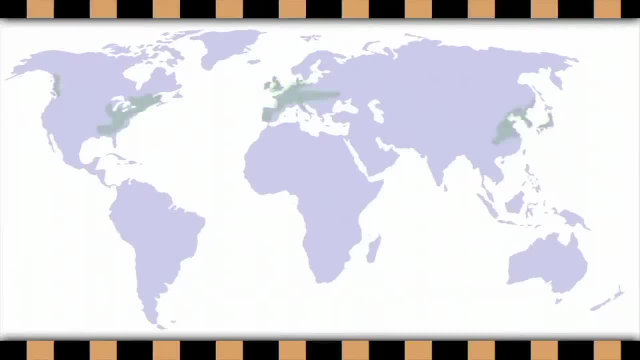 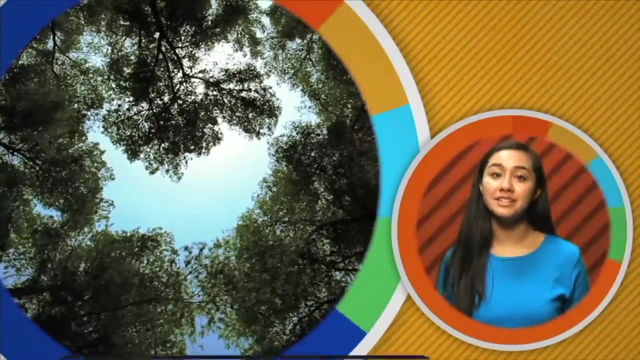 the deciduous forest. The deciduous forest regions exist in many places, including eastern North America, Europe and eastern Asia. What makes this forest so different? Well, it has mostly deciduous trees, trees that lose their leaves during the autumn season. 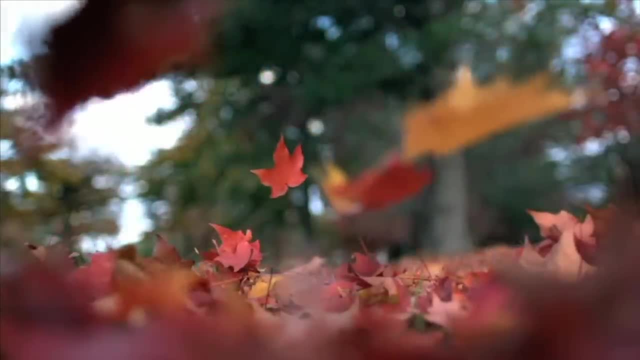 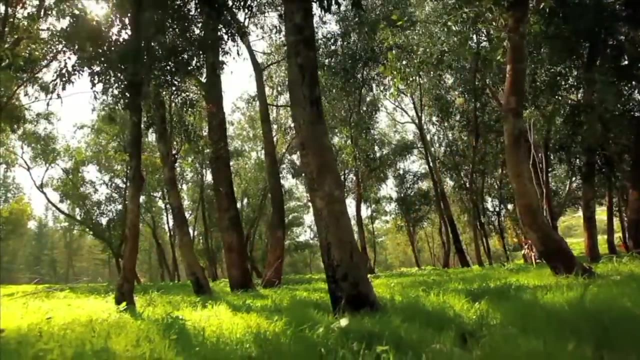 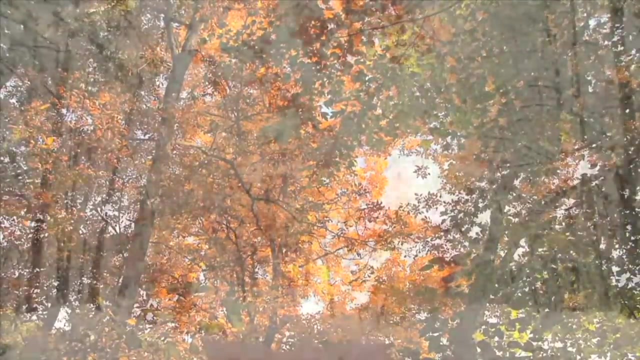 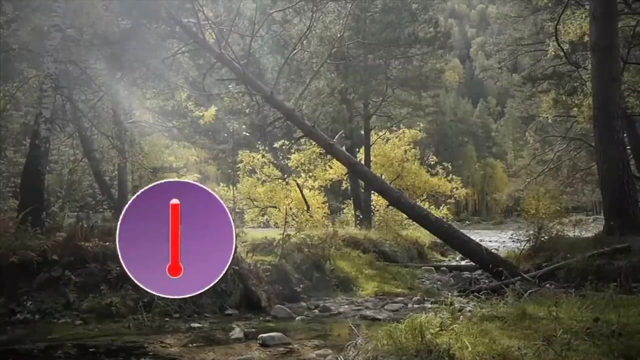 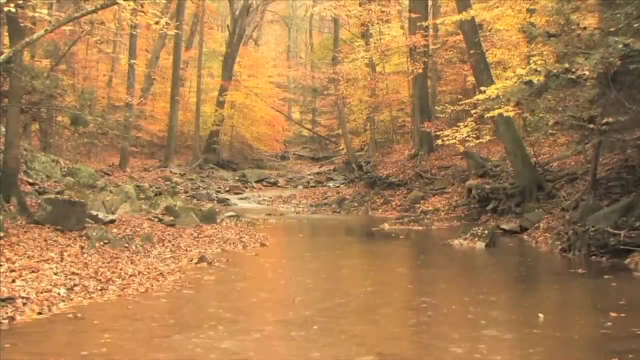 The decaying leaves make the soil very fertile and, as a result, this biome can support all different kinds of plants and animals. The climate here changes, and the forest experiences all four seasons: summer, autumn, winter, spring. The deciduous forest has an average temperature of 10 degrees Celsius, and rainfalls add an. average of 75 to 150 centimeters annually. So you can find a wide range of animals that live in this biome: Deer, squirrels, rabbits, chipmunks and even people, Because the soil is so fertile. many people have read areas of the deciduous forest to 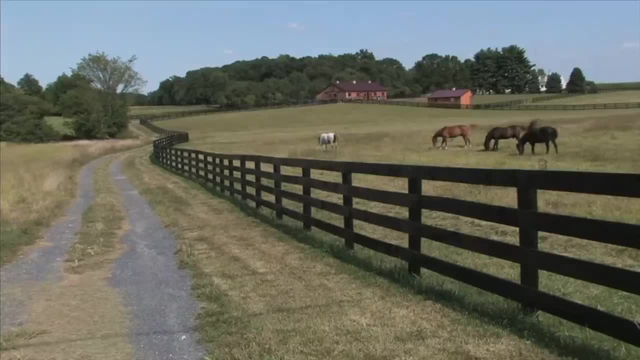 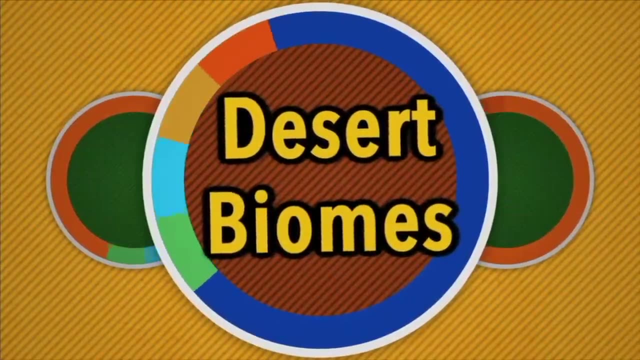 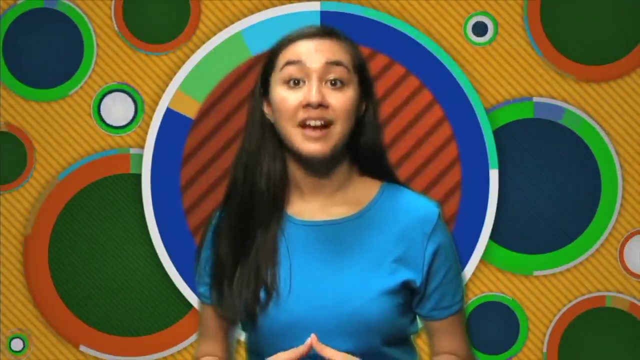 create homes and farms there- Desert Biomes. Let's move on to a biome where it's difficult for life to survive: The desert. Scientists estimate that about one-fifth of land is a desert In different times of the year. this biome is called the desert biome. 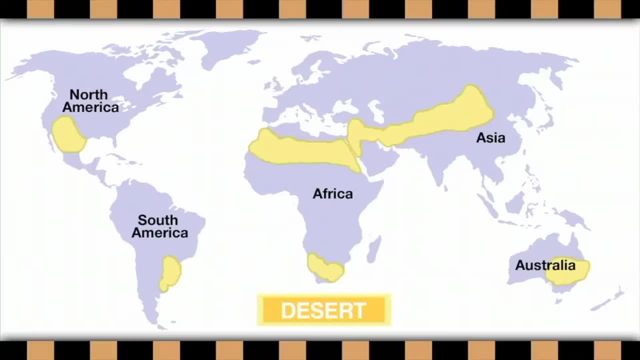 The desert biome is called the desert biome. Scientists estimate that about one-fifth of land is a desert. In different times of the year, about one-fifth of land is a desert. Types of deserts can be found on virtually every continent except Europe. 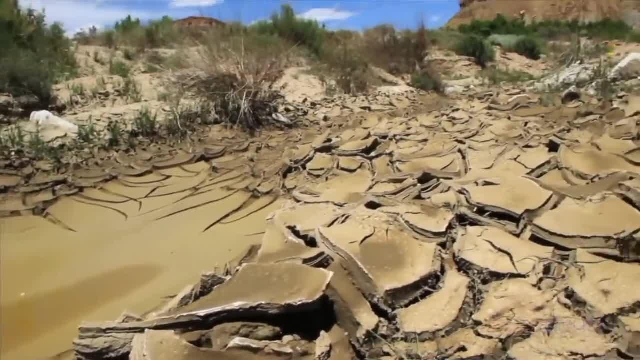 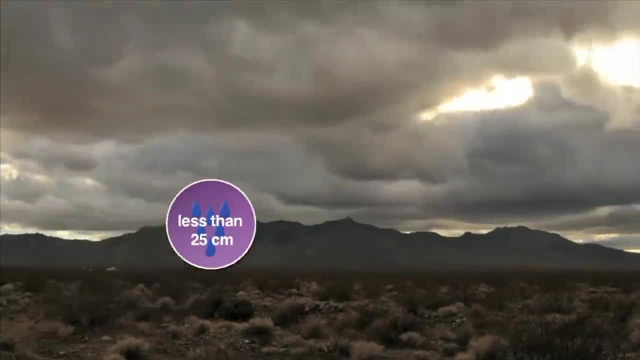 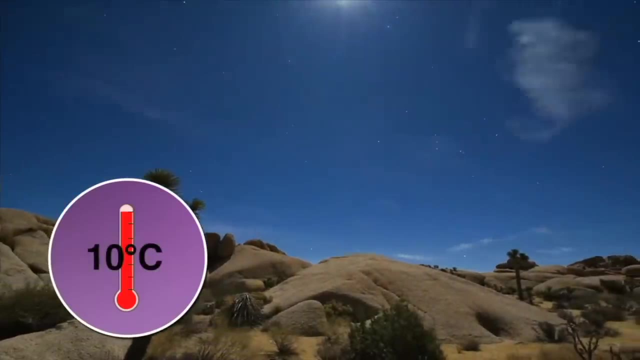 This biome can support very little life because of the lack of water. Average rainfall in the desert is less than 25 centimeters per year. Temperatures range from about 35 degrees Celsius during the day to 10 degrees Celsius at night. Desert Biomes. 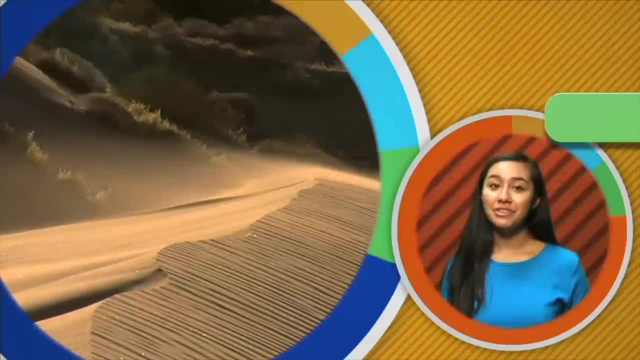 The desert biome is a biome that can be found on virtually every continent except Europe. Types of deserts can be found on virtually every continent except Europe. This biome can support very little life because of the lack of water. Temperatures range from about 25 square meters to 13 frames per second. 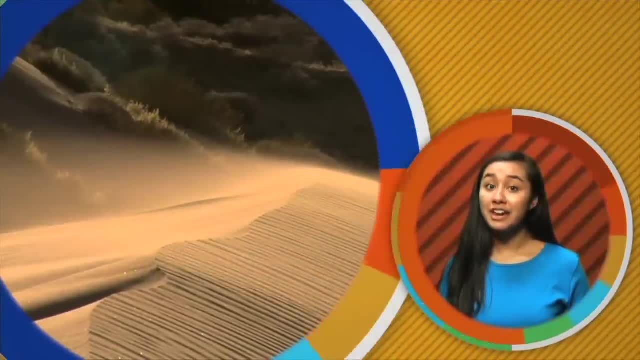 This biome is a biome that can support very little life because of the lack of water. When you think of a desert, you might think of a very hot, dry place, But there are actually different types of deserts with different climates. One kind is hot and dry. 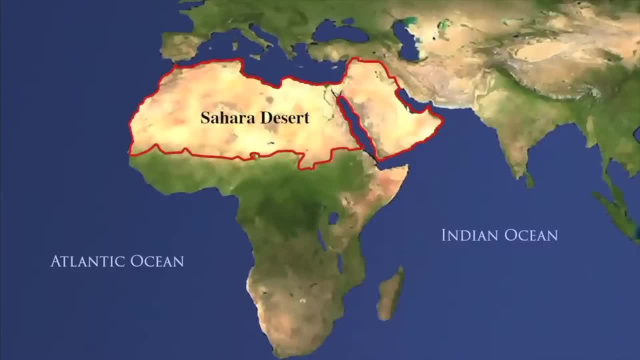 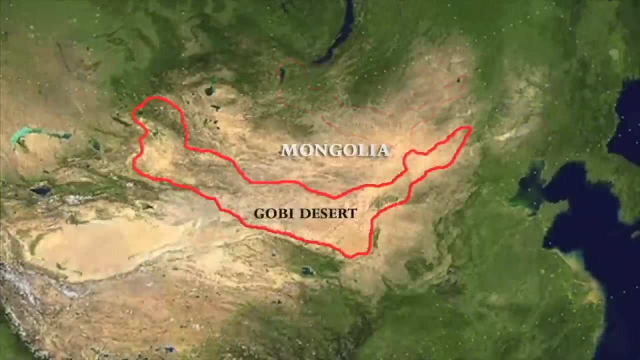 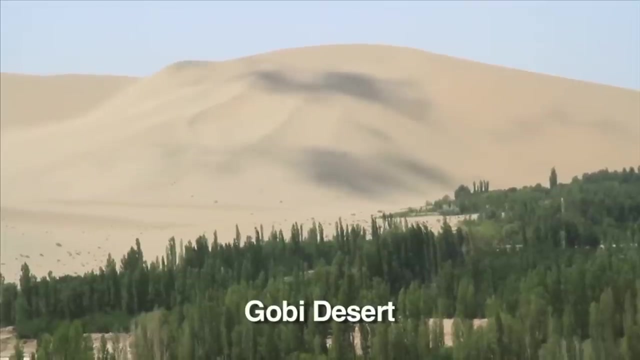 An example of a hot dry desert is also the world's largest desert—the Sahara in Northern Africa. It stretches across almost 9.1 million square kilometers. Another kind of desert is cold and dry… The Gobi Desert in northern china. this desert stretches across almost 1.2 million square kilometers. 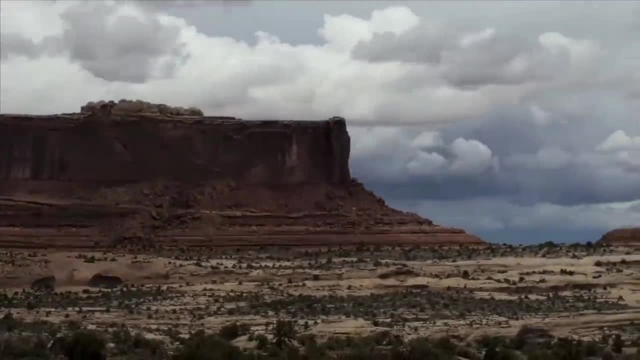 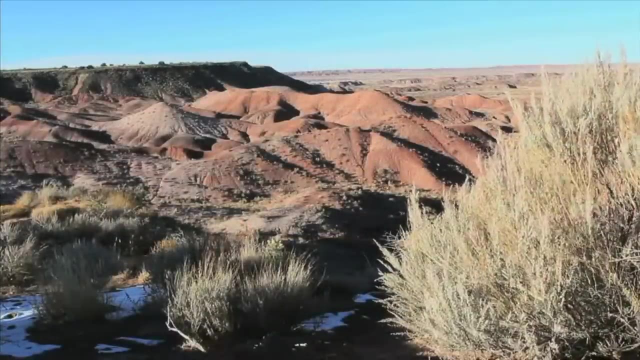 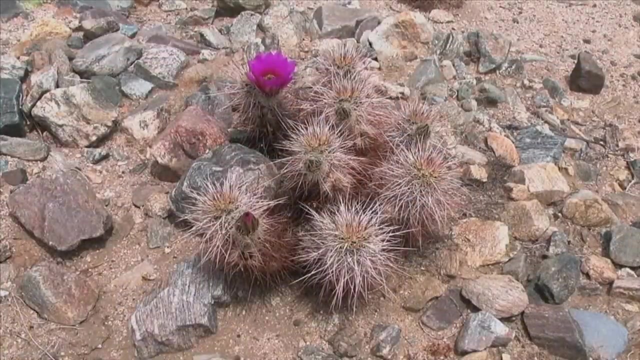 each type of desert has its own plants and animals, all of which have adapted to low moisture conditions. in the cold, dry desert, plant life is scarce, and so are the animals. in the hot desert, you can find many different cactus species and some other types of plants. 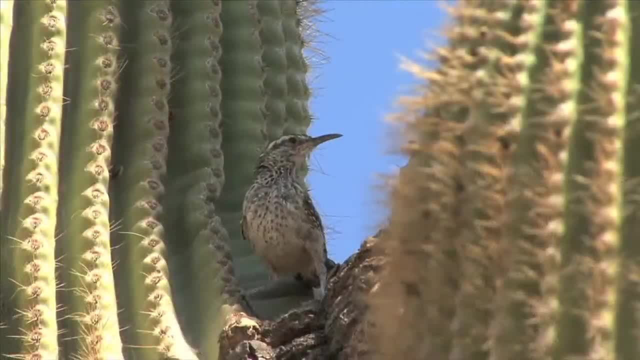 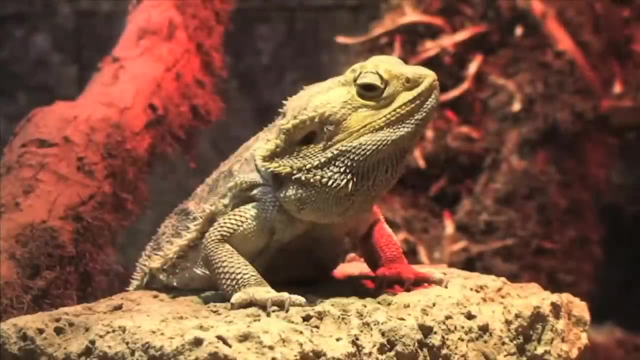 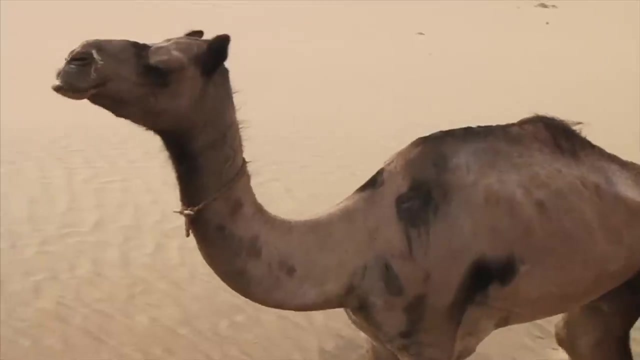 few animals are equipped to survive here, but there are a variety of reptiles, including snakes and lizards, and let's not forget the camel. it can survive in these dry conditions by storing water, producing fat in its hump, and it can also be used as a food source for other animals. 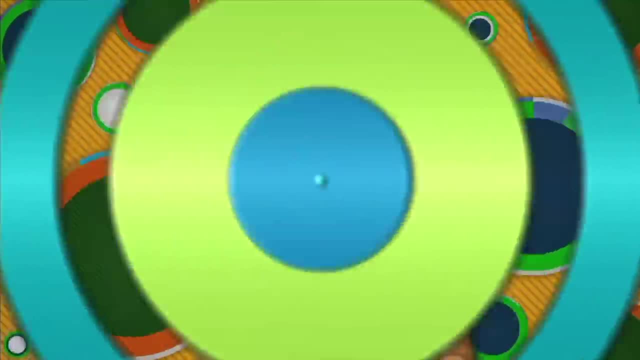 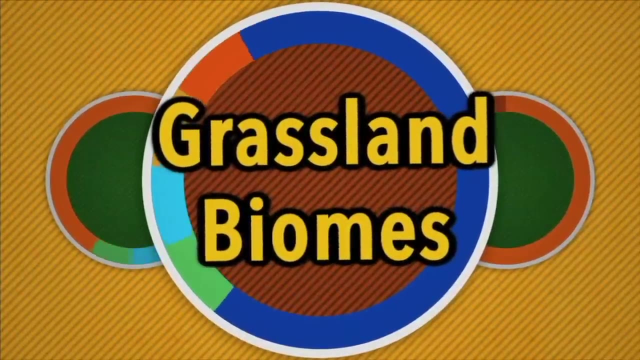 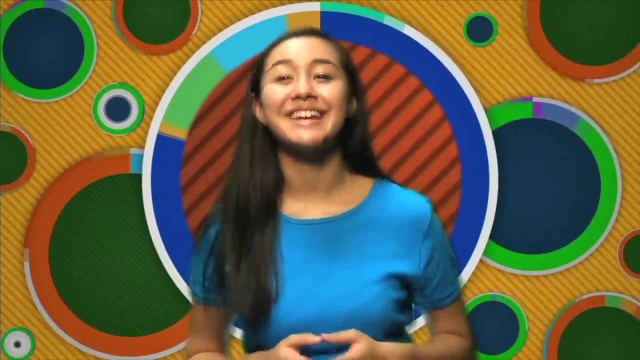 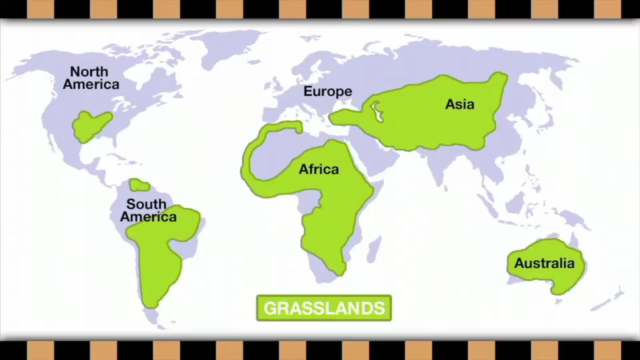 ready to move on to another region, here we go: grassland biomes. this biome is called the grasslands and it's full of- you guessed it- grass. grasslands can be found in virtually every continent. it's estimated that almost one quarter of land is grasslands. 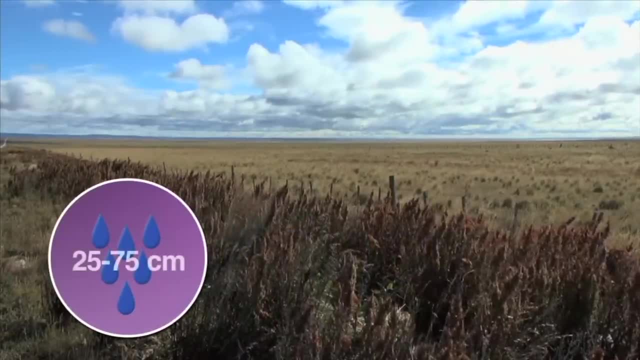 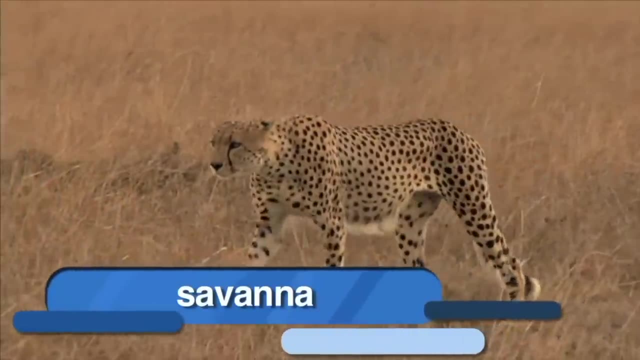 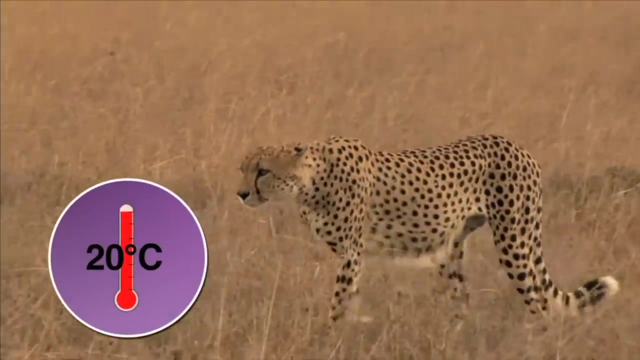 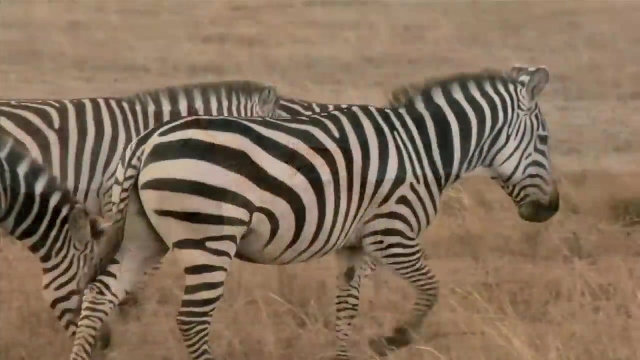 and there are different kinds of grasslands, each of which see an average of 25 to 75 centimeters of rainfall annually. temperatures in the savannah, which is the hot tropical grassland found in africa, very little and average about 20 degrees celsius. there you'll find mostly dry grassy fields and animals like giraffes and zebras. 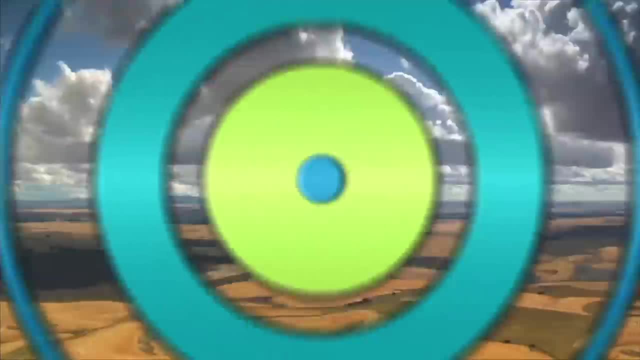 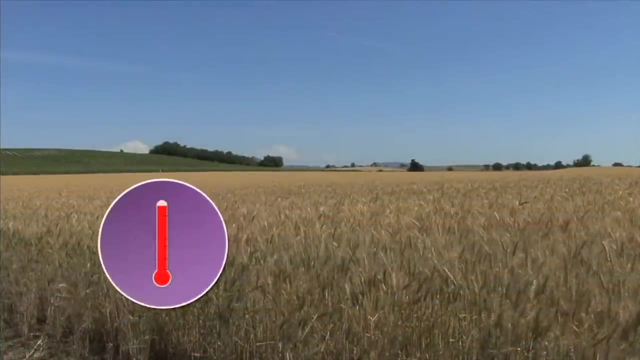 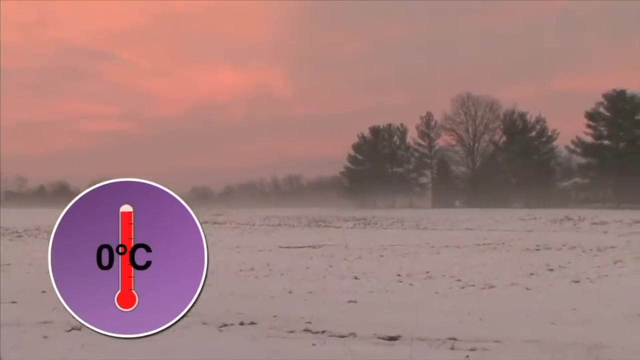 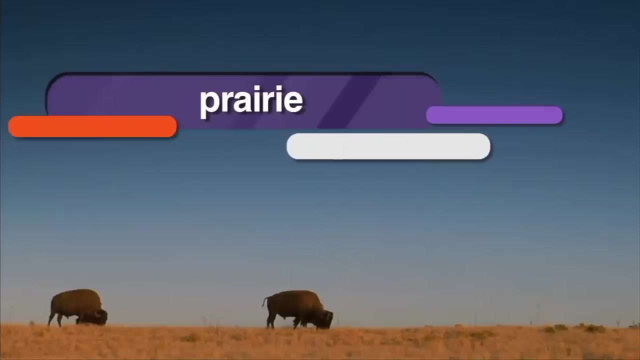 There are temperate grasslands too, like the ones found in North America, which have a varying climate, with temperatures ranging from 38 degrees Celsius in the summer to zero degrees Celsius in the winter. These grasslands are often called prairies and are home to animals like buffaloes and 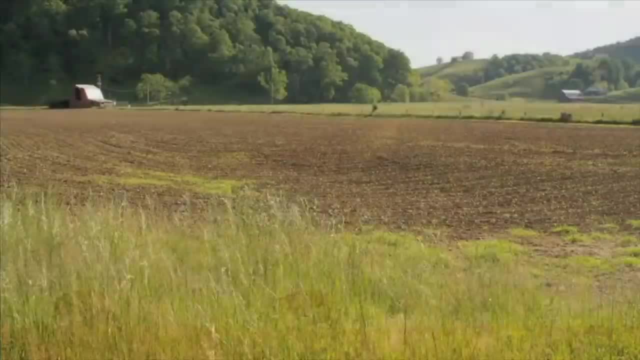 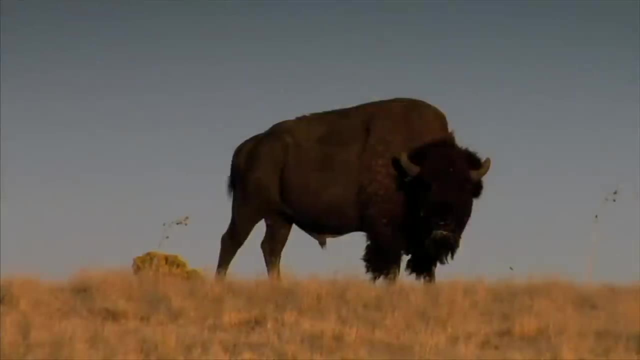 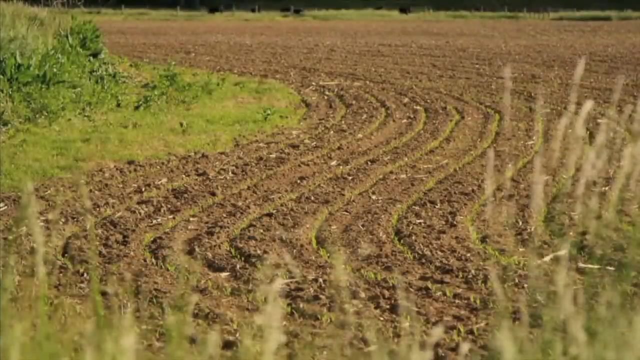 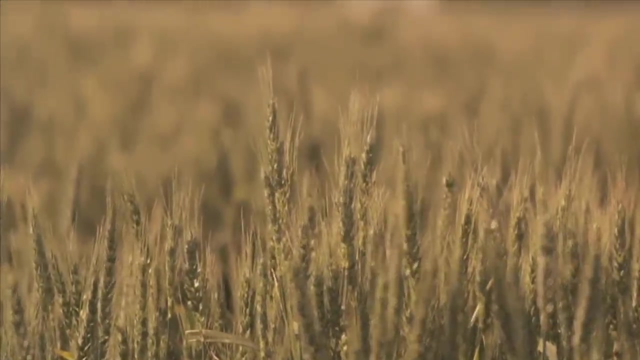 prairie dogs. In many places in North America and Africa, grasslands have been turned into farms, making it less likely for large wild animals like bison to live there. The nutrient-rich soil is great for raising crops and feeding animals. So much of the grasslands are used for food that the area in the United States is often 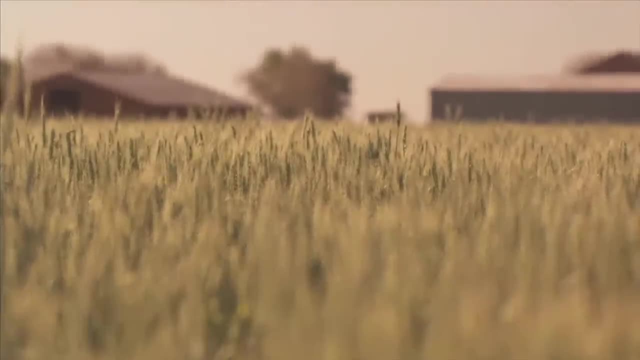 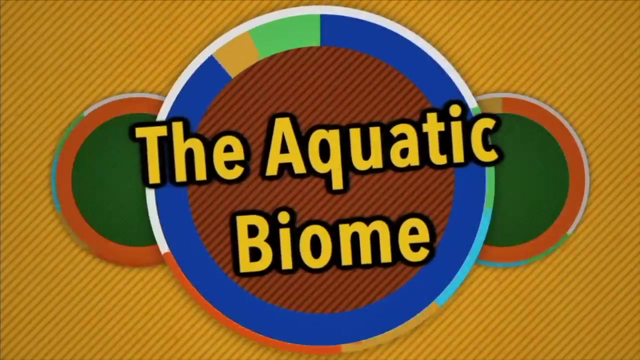 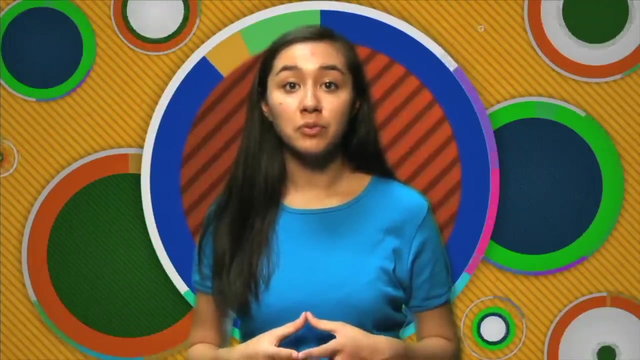 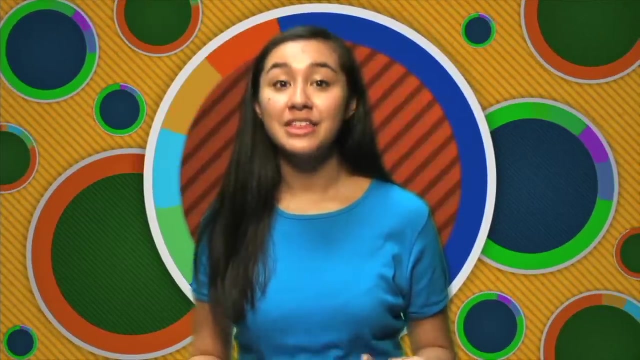 called the breadbasket of America. さて便はどうなるんですか؟? The Aquatic Biome. Moving on from the rolling hills of the grasslands, we come to a biome that covers approximately 75 percent of the earth's surface-the Aquatic Biome. 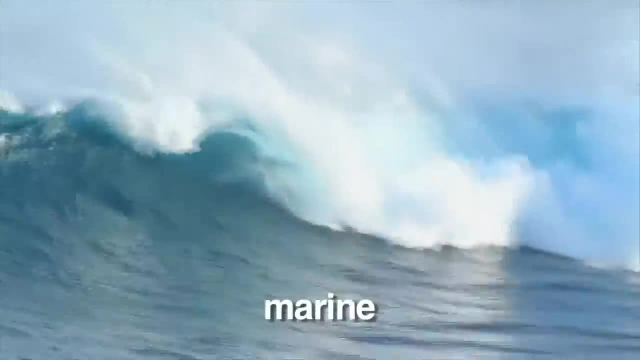 This biome can be separated into two basic regions-marine and fresh water. The basic biome is the Aquatic Biome, the biome of fertile soil with an active biome. The biome is the biome that is alimented by the aquatic system. The biome is the biome of freshwater and freshwater. 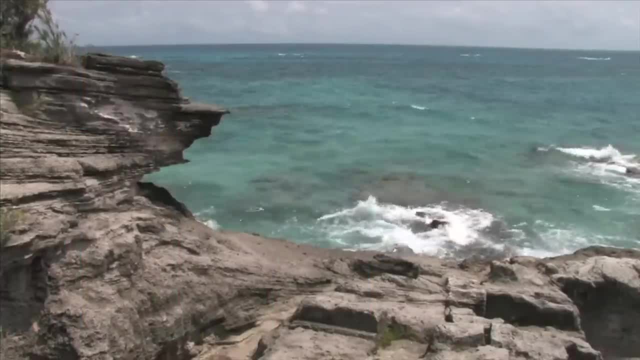 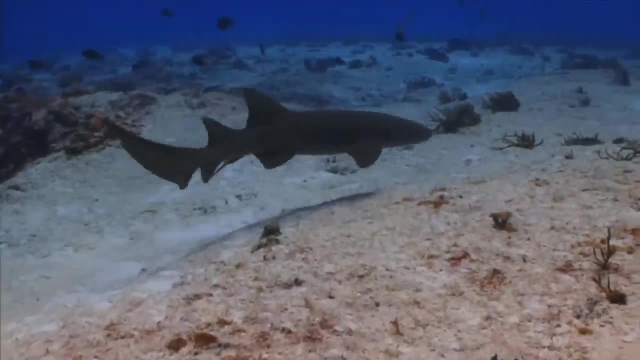 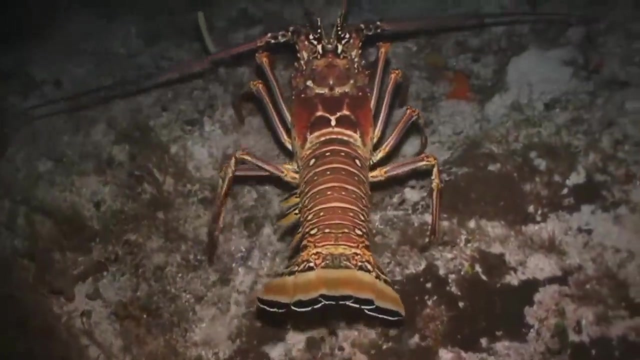 It is the biome of all. the water in the ocean include bodies of salt water such as oceans and some lakes. Marine regions support all kinds of animals, including sharks, fish and seahorses, as well as crustaceans and mammals like dolphins. Seaweed makes up a large portion of the marine plant life. Now, fresh water regions are made up of fresh water, not salt water, and includes ponds, lakes, streams, rivers and wetlands. The various freshwater regions are home to many different types of animals, like fish, beavers. 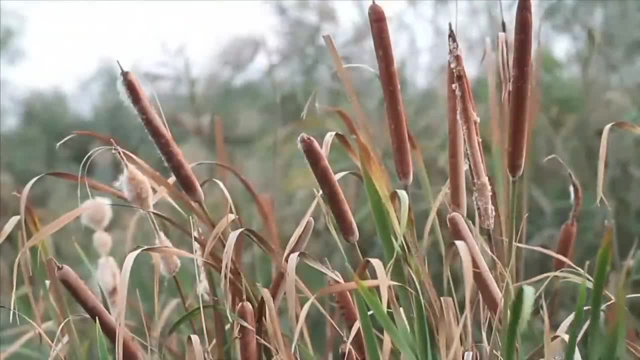 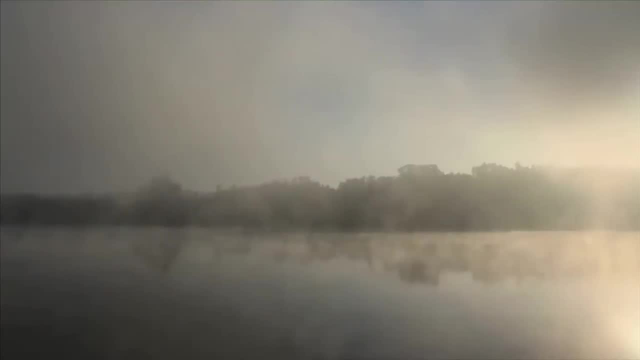 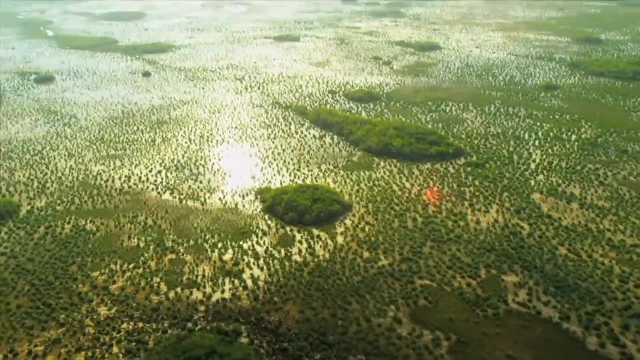 and ducks, And different kinds of plants can be found in the different freshwater regions. Temperatures can vary widely among the aquatic biome regions depending on location, but generally these areas tend to be more humid and have a cooler air temperature than terrestrial biomes. 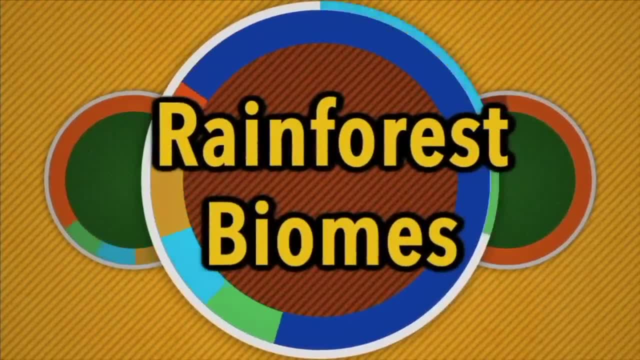 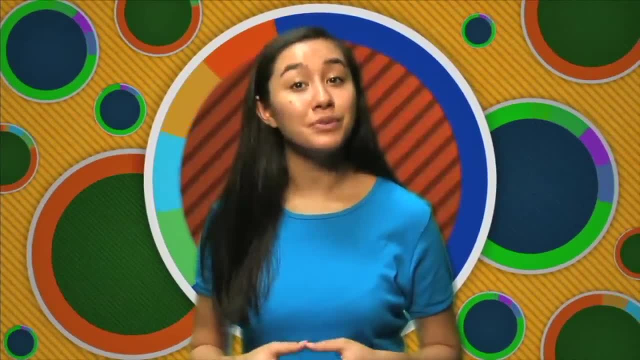 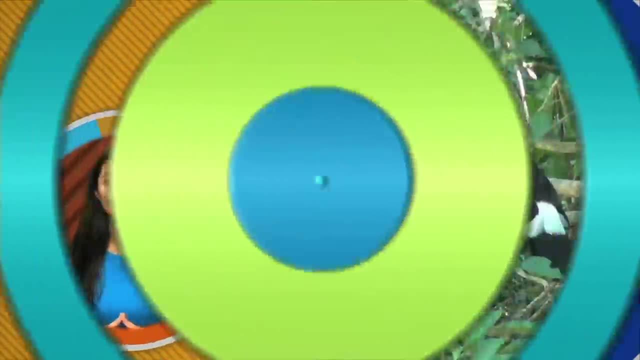 Rainforest biomes. That brings us to the last major biome we're going to discuss, and it's one of the most interesting. It's called the rainforest and it is home to almost half of all the world's plant and animal species. There are two basic types of 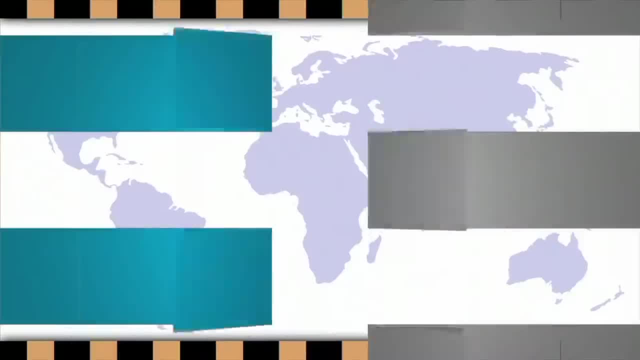 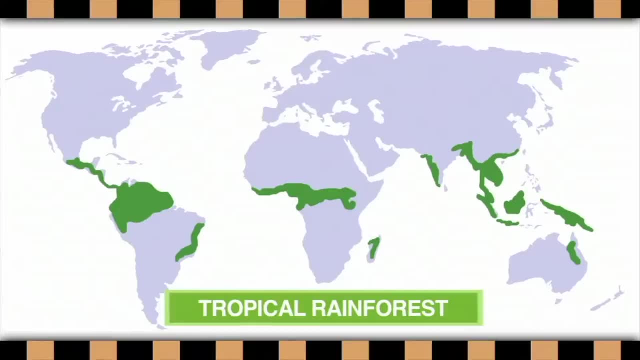 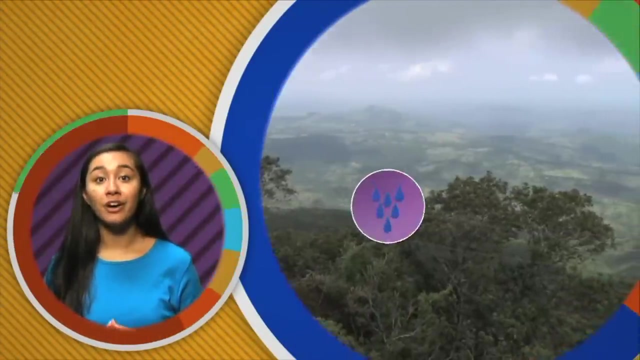 rainforests. tropical and temperate Tropical rainforests can be found in Asia, Africa, South America, Central America and many islands, many near the equator. Now, the largest temperate rainforest can be found on the Pacific coast. Tropical rainforests can get up to 400 centimeters of rain.